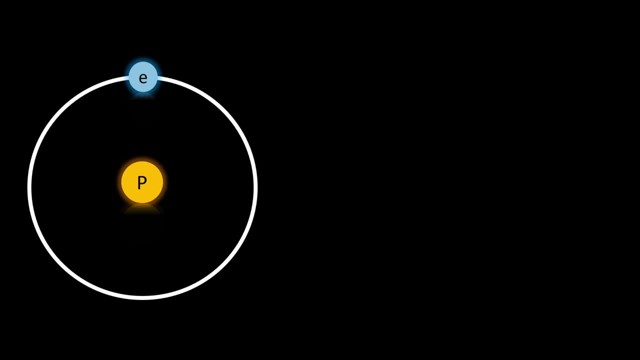 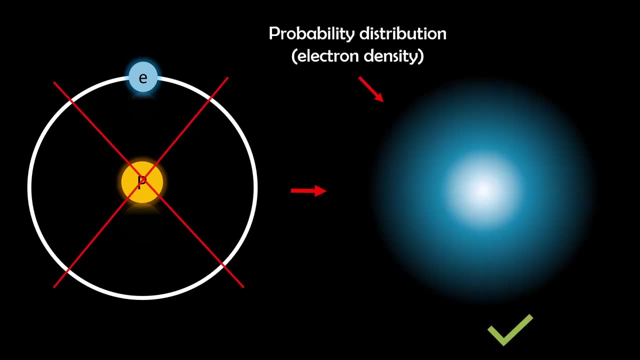 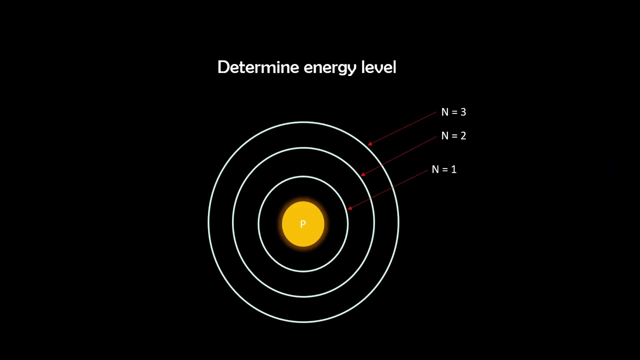 The Schrodinger equation helped our understanding of electrons. Rather than pinpointing an exact location, the equation allows us to map out the electron densities, as well as determine its quantized energy level, And solving these electron densities are how we get atomic orbitals, which are 3D regions of space where electrons are most likely. 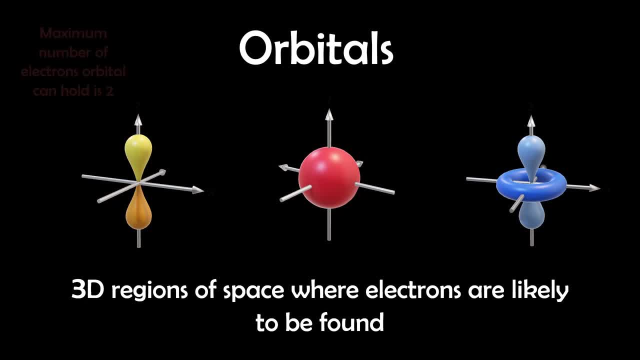 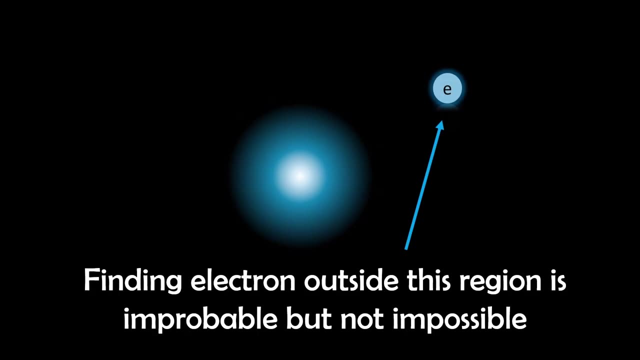 to be found. Each orbital can host up to two electrons, and these orbitals only exist if they are occupied by electrons. They are energetically favourable locations for electrons, so finding an electron outside these orbitals is highly improbable due to electron energy. 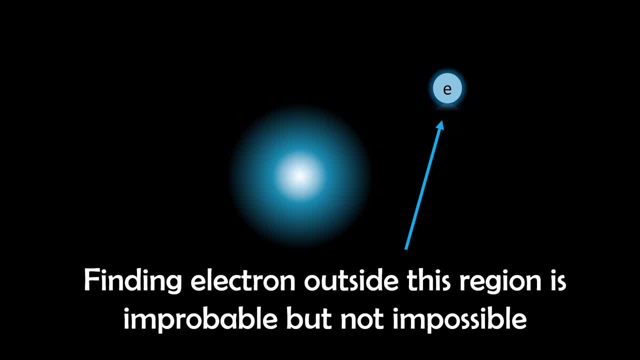 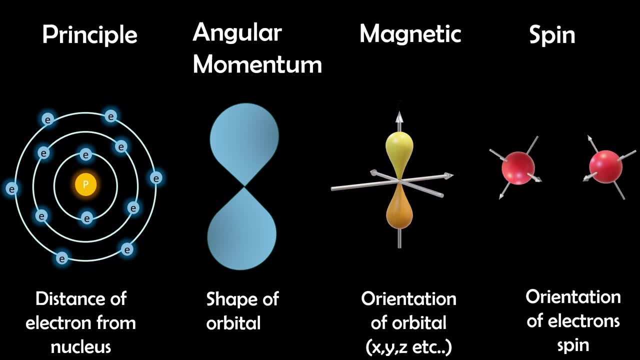 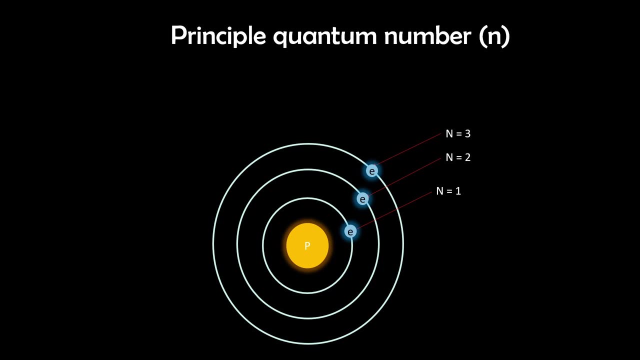 constraints, but it's not impossible. The behaviour of electrons in these orbitals is described by four quantum numbers. The principal quantum number n is any positive integer, so for example 1,, 2,, 3,, 4, etc. and. 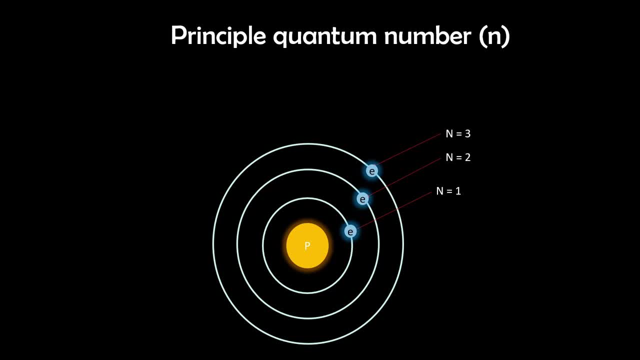 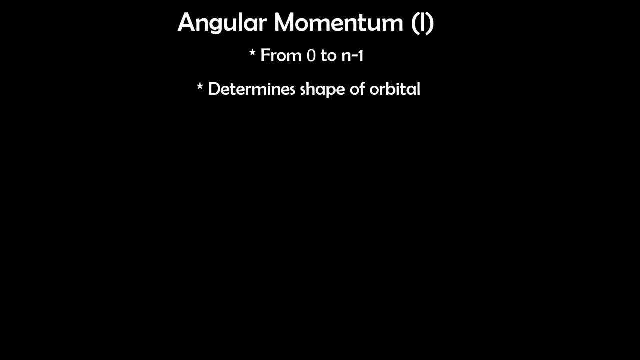 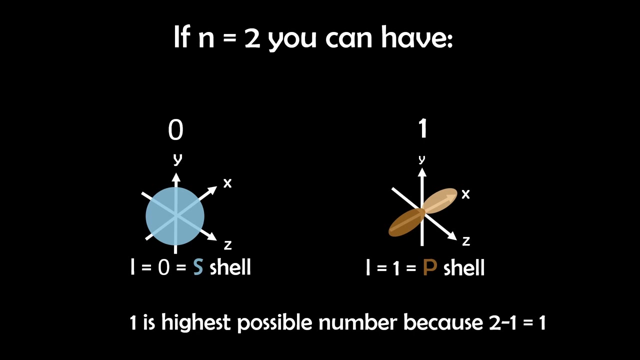 it indicates the electron's energy level relating to its distance from the nucleus. This concept was initially introduced in the Bohr model, so these distances represent principal quantum numbers. The next is the angular momentum quantum number, or n. The angular momentum quantum number, or n, is: 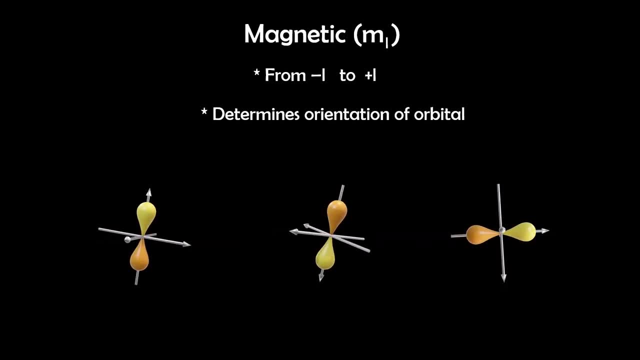 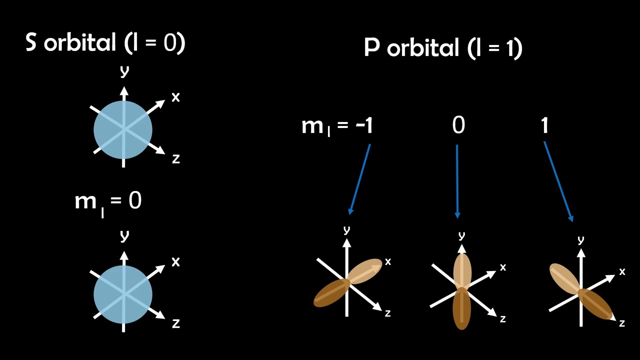 The magnetic quantum number m sub L, which can be any integer between negative L or positive L, specifies the orbital's orientation. This number relates to the possible configurations of each orbital shape. For example s orbitals where L equals 0 only have one configuration, so m sub. 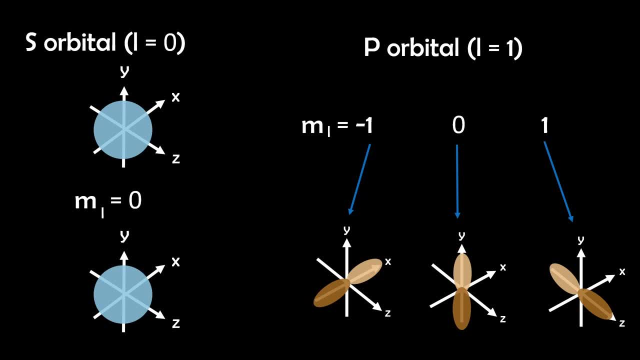 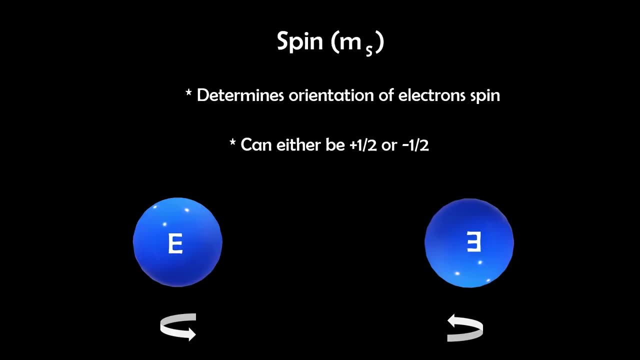 L equals 0,, whereas p orbitals, where L equals 1, have three configurations where m sub L can equal negative 1,, 0, or 1, and so forth. Lastly, the spin quantum number m sub s, which is either: 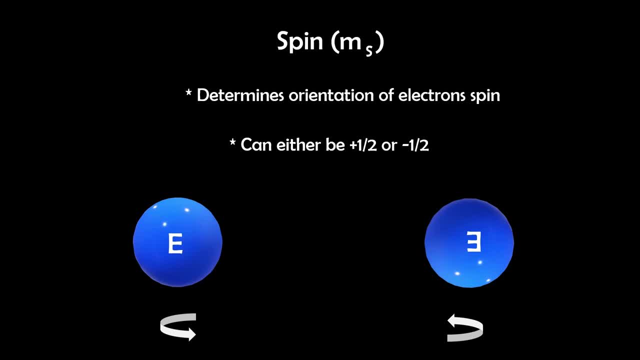 positive half or negative half represents the electron's spin direction. This aligns with the Pauli exclusion principle, ensuring no two electrons are in the same direction. In other words, no two electrons in an atom have the same set of quantum numbers. 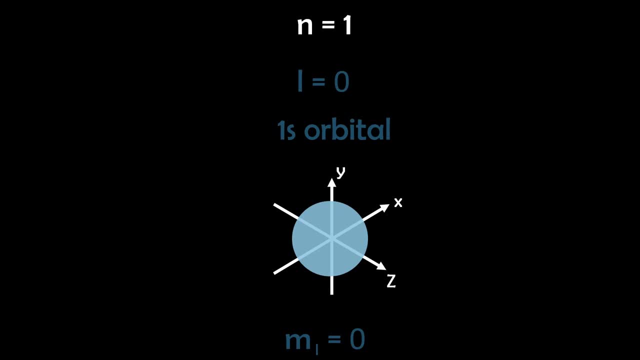 Now let's look at some quantum numbers. For n equals 1, the simplest level we encounter, the 1s orbital. Here L equals 0 and m sub L is also 0, indicating it's a spherical orbital with room for two electrons of opposite spins. It's the lowest energy orbital, making it 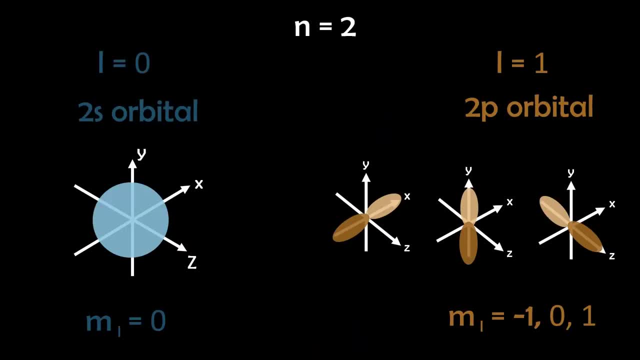 the first to be filled, Moving up to n equals 2,. we have two types of orbitals: The 2s, where L equals 0, and 2p, where L equals 1.. The 2s orbital, similar to the 1s orbital, has a spherical shape. 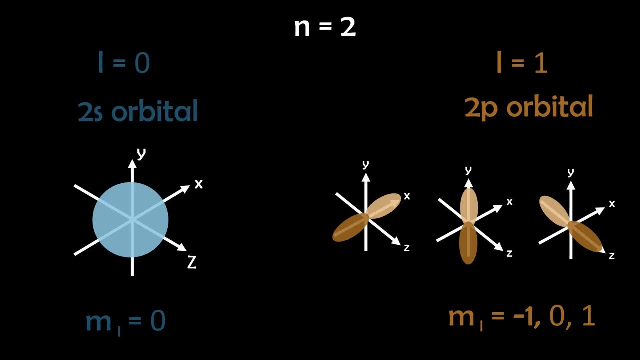 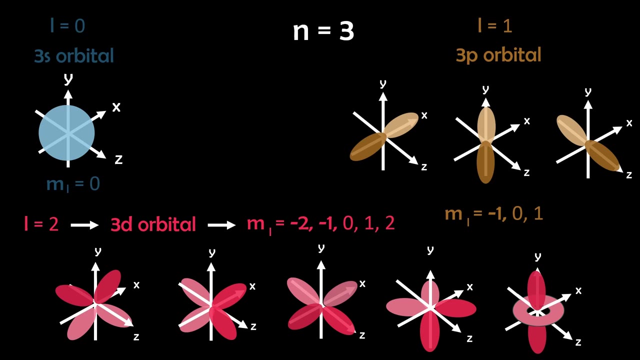 But the 2p orbitals are more complex, with m sub L values of negative 1,, 0, and 1,, each capable of hosting two electrons. Thank you. At the n equals 3 level, things expand further. We see the 3s orbitals where L equals 0,. 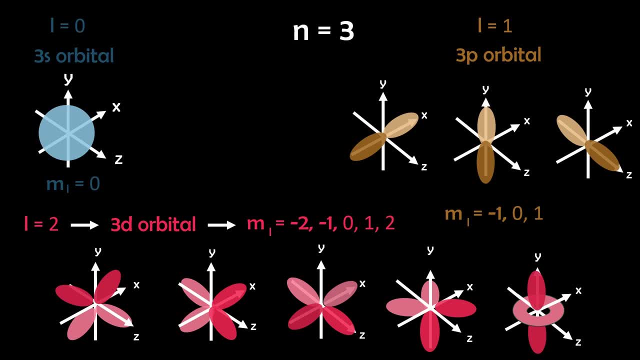 and the 3p orbitals, where L equals 1, with three possible configurations. Here the orbitals increase in size and energy. But we also encounter the 3d orbitals, where L equals 2,, which represents five unique configurations reflecting more ways electrons can be arranged. 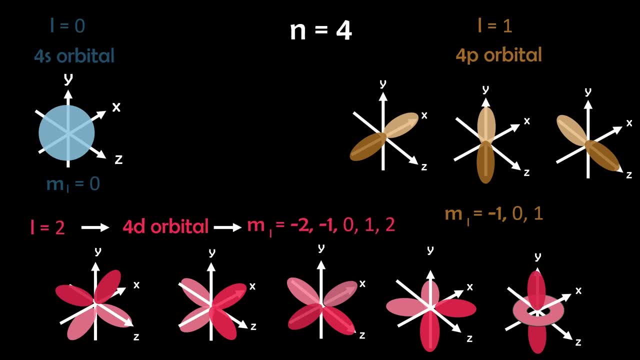 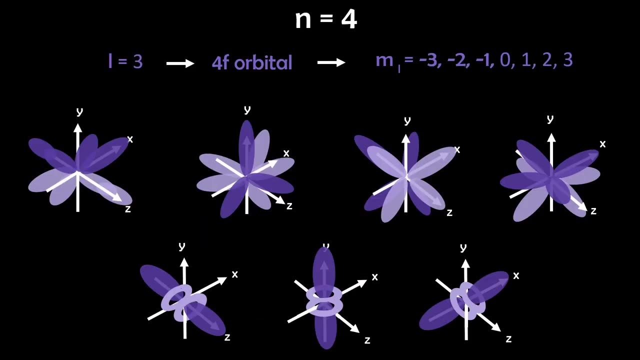 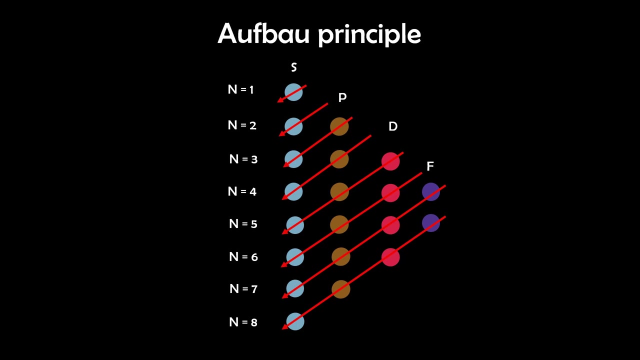 For n equals 4, the orbitals look even weirder. Electrons can occupy the 4s, 4p with three configurations, 4d with five configurations and finally 4f orbitals which have seven configurations. The sequence in which these orbitals are filled is guided by the Alfebel Principle, a topic 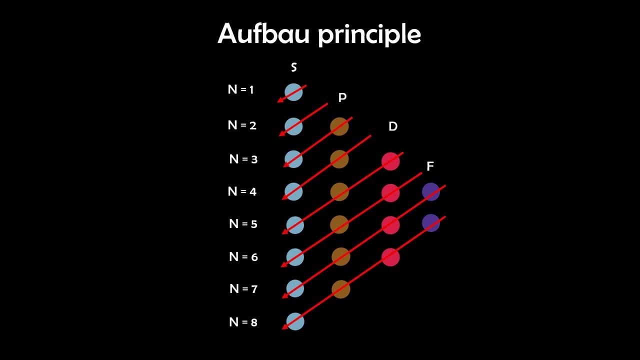